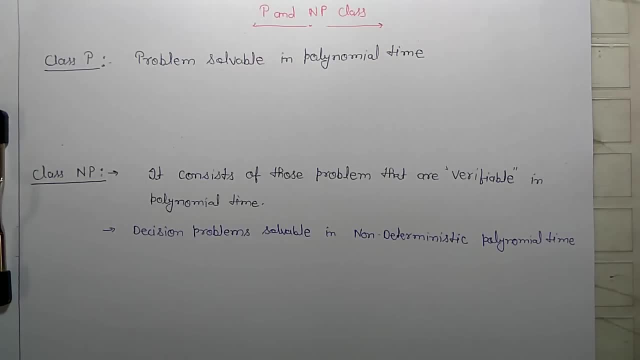 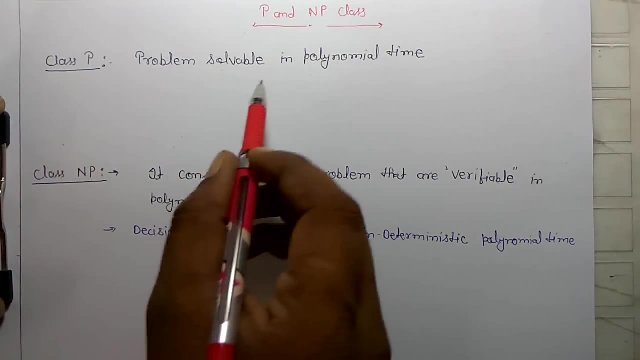 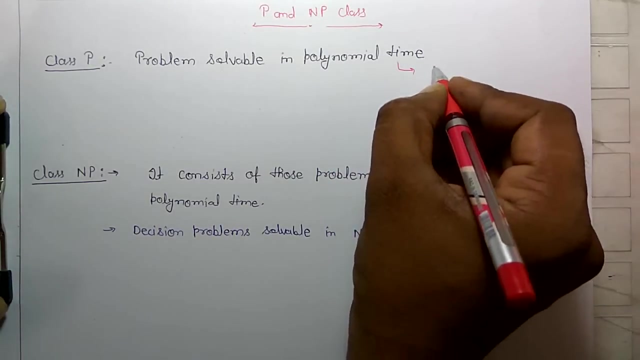 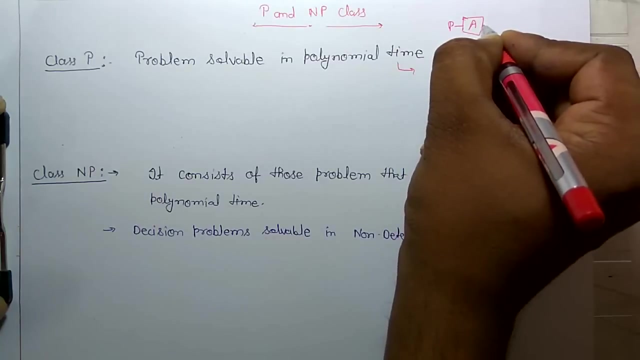 Hi, today we are going to learn P and NP class problem. So the class P problem means the problem that can be solved in polynomial time. So what is polynomial time? It means if there is algorithm that solves a problem- P and gives some output, and the algorithm complexity. 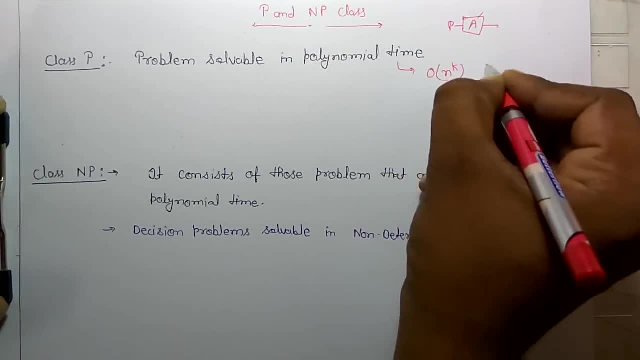 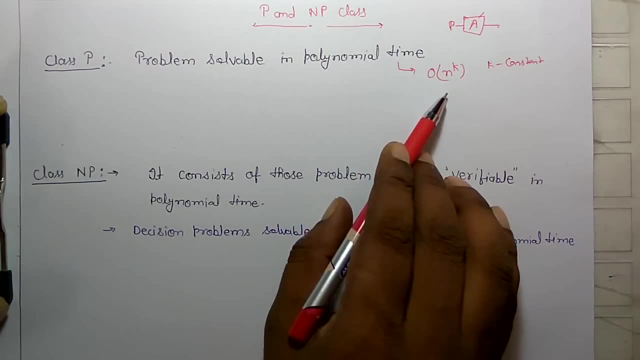 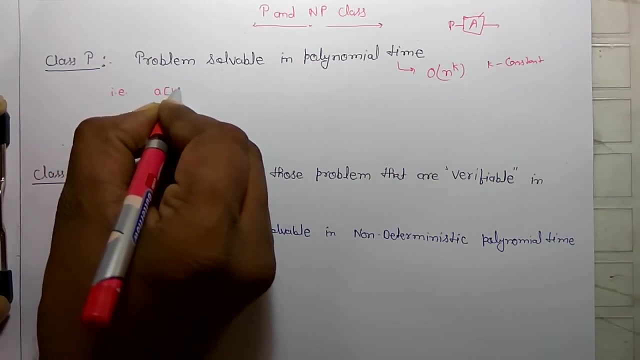 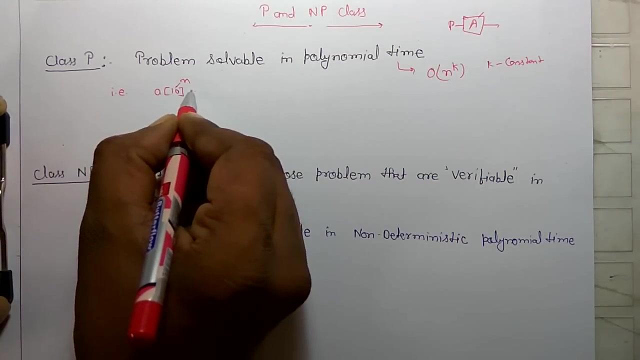 is O of n power k, where k is constant value. So that is polynomial time. So in any problem, for example, if there is array A of 10 or it can be considered as n size of n and you have to find element x where it exists in this array or not. 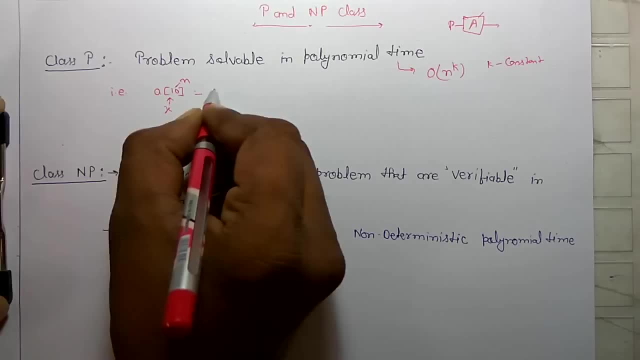 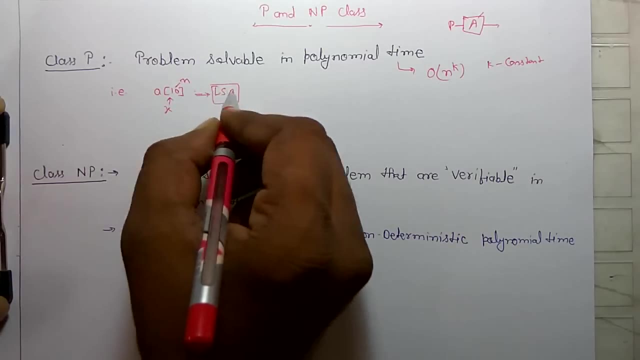 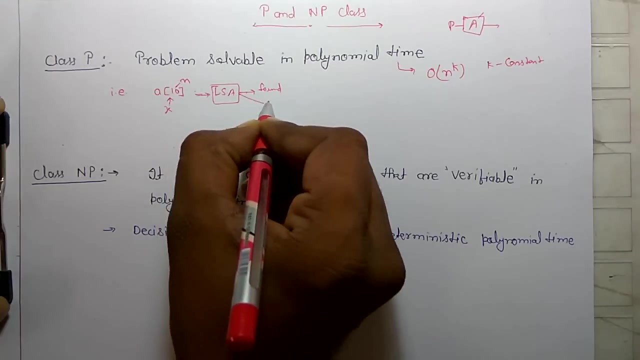 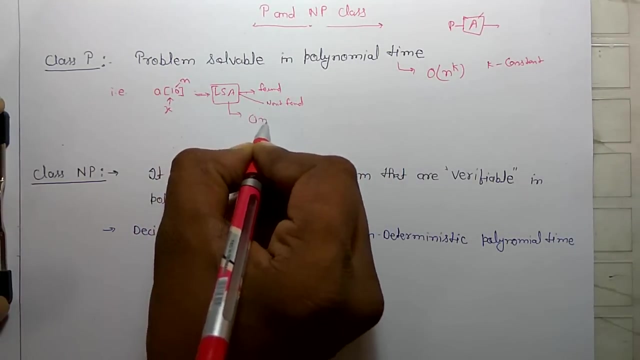 So for this problem you have created a linear search algorithm. You create a linear search algorithm and you can find this problem by using linear search algorithm. This is found or not found, X is found or not found, And the complexity of this linear search algorithm is O of n, So it is P class problem. 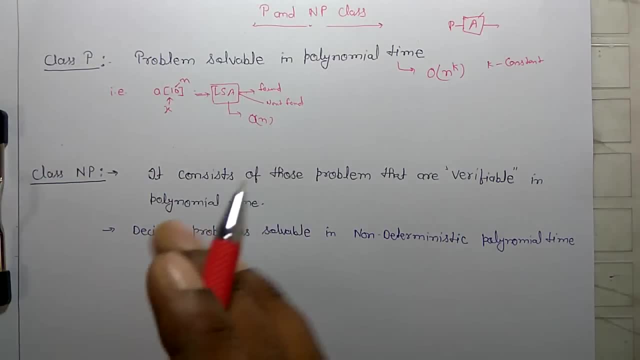 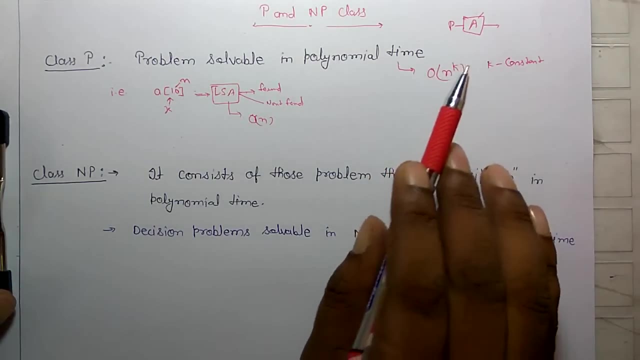 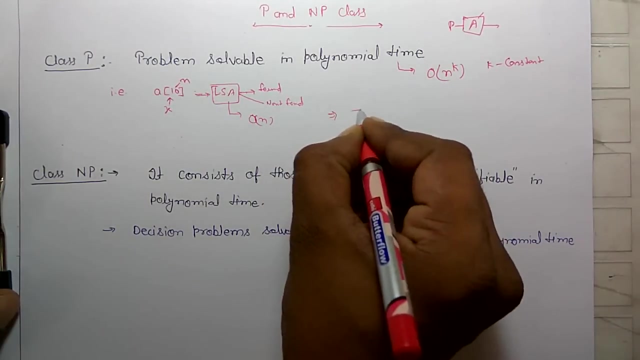 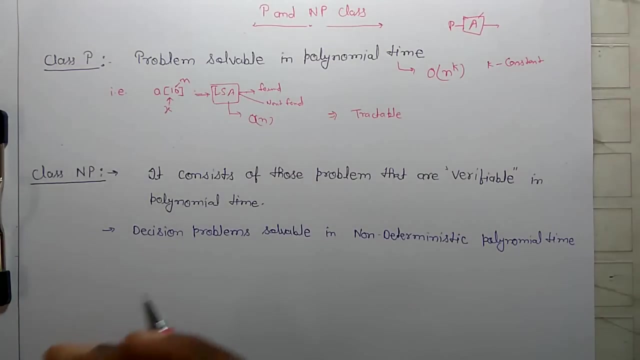 So what is P class problem? The algorithm solves that problem in polynomial time. So this is polynomial time, And if any problem is solved in polynomial time, that is also tractable problem. Tractability and intractability are two terms used in P and NP class. So what is tractable problem? 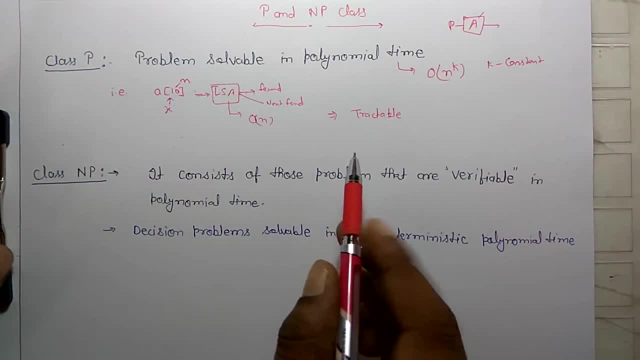 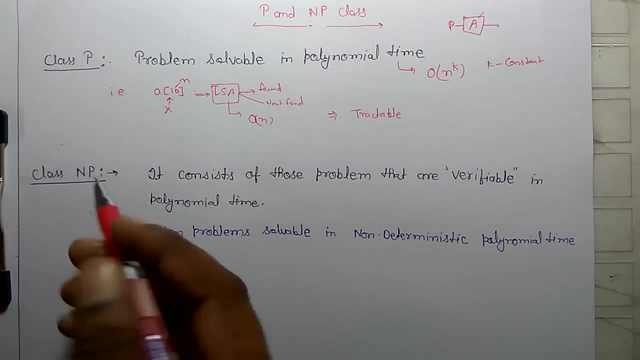 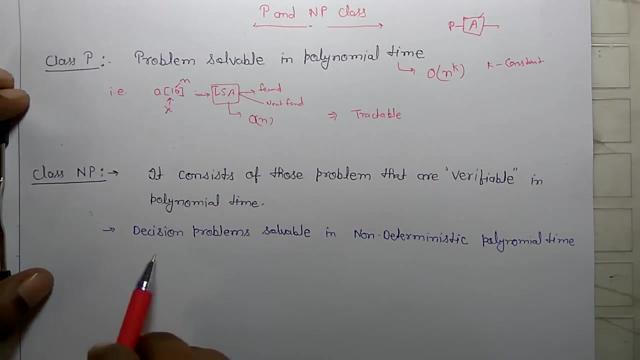 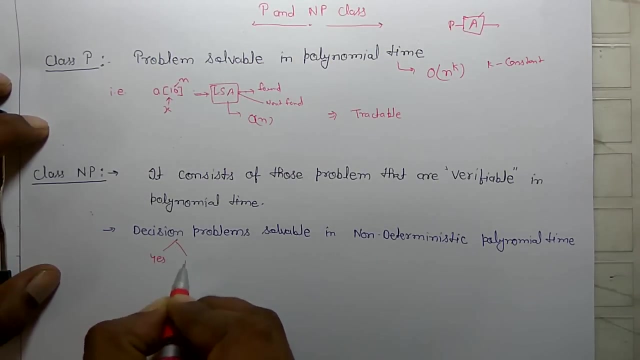 The problem is solved in polynomial time, And what is not solved in polynomial time, that is also tractable problem. So next class is NP class. It means there are some problems that cannot be solved in polynomial time. So the decision problems. decision problems means the answer can be given in yes or no. 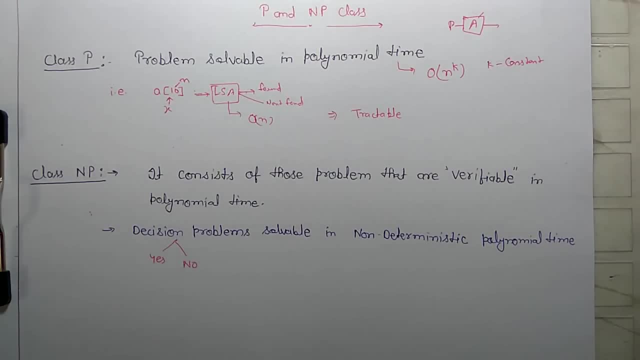 The decision problems solvable in non-detachable form. The solution can be solved in non-deterministic polynomial time, So it should be solved in polynomial time, but not in non-deterministic polynomial time. So what is deterministic and non-deterministic? 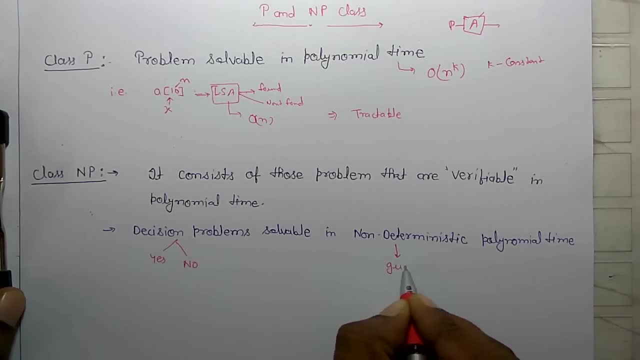 In non-deterministic, you perform. guess Through guess you find the solution. For example, there is a Sudoku and you have to solve it. So you perform some guesses And through brute force, you solve this Sudoku. It may take exponential time. 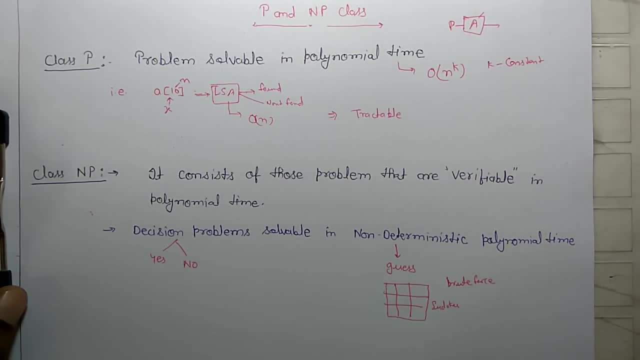 So this Sudoku can be solved or not solved, That you can verify it. There is some solution through which you can verify that this, the solution you have given for the Sudoku, Is correct or not. So what happens in NP class? It consists of those problems that are verifiable in polynomial time. 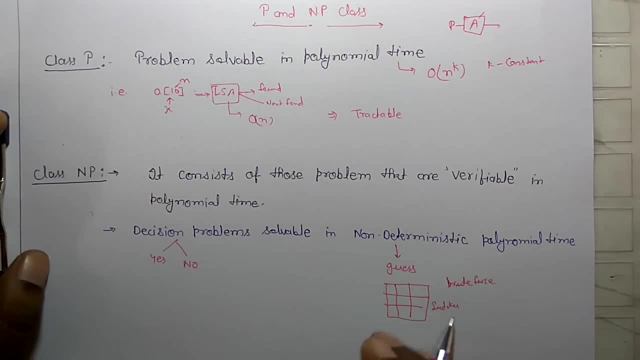 Means you have found the solution of any problem through brute force. However you have found it. But what you have found, that was very difficult. You guessed that you can keep 9 here. you can fill 8 here In Sudoku solving, But when it is solved, 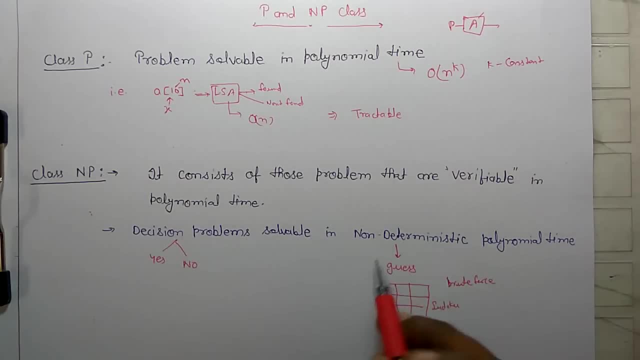 You said that this is solved, So any other person can verify it. There is some logic through which you can easily verify it And obviously that person will take less time in compared to solving your problem. So that class of problem goes into NP class. 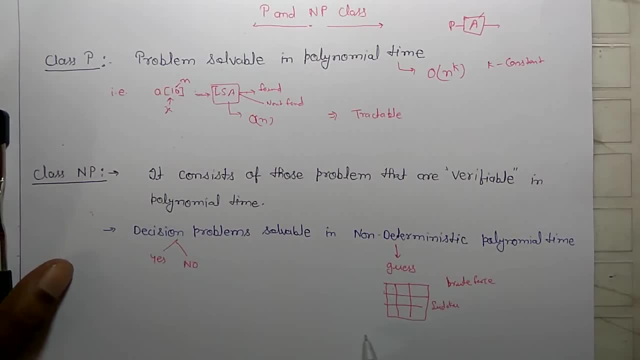 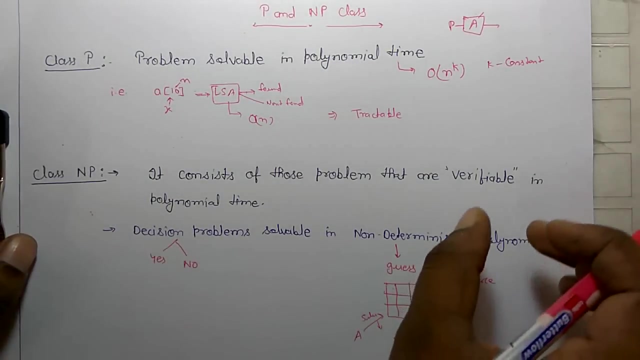 Okay, Means if any person has solved this Sudoku And he invested some time, But there is a, B, another person that can verify In very little time In compared to A who solved it. So what will happen in NP class? There is a verifiable? 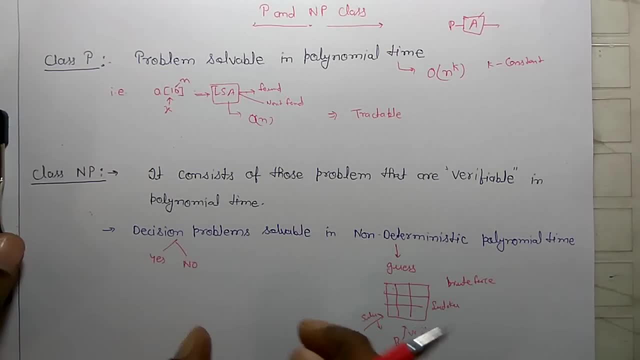 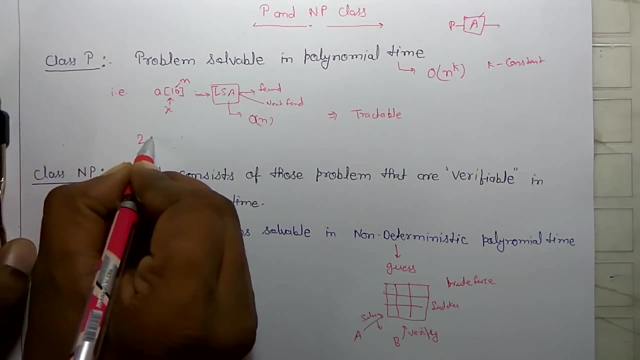 Means there will be a certificate solution Through which you can verify it. What are its examples? Like 3 set problem- Okay, And 3 CNF problem. This is from Boolean algebra. 2 CNF is your P class problem. 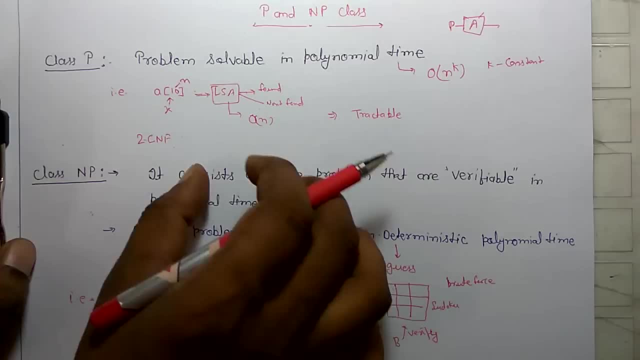 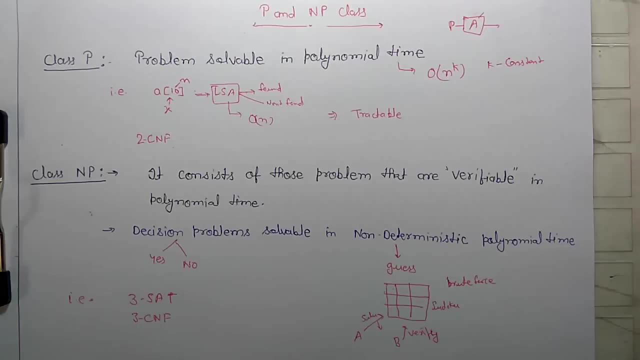 So if there are 2 variables And it has CNF representation, Then you can verify Whose answer will be true and whose answer will be false In polynomial time. In NP class there is some problem like TSP Travelling cells problems. 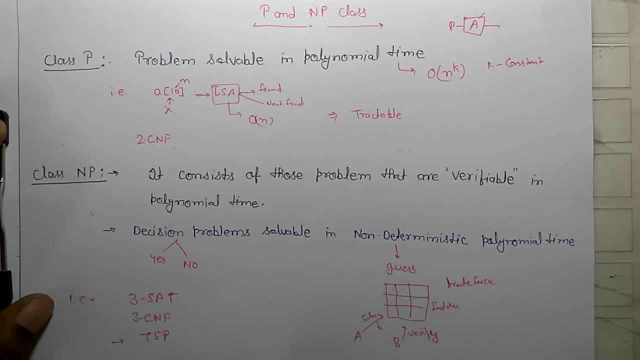 So if there are a lot of nodes, Then in that you have to find Travelling cells problems solution. So that exists in NP class. If you remember the knapsack problem, What was in knapsack problem? That we had some bags. 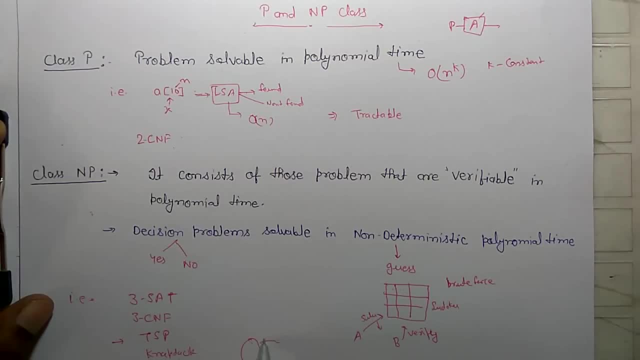 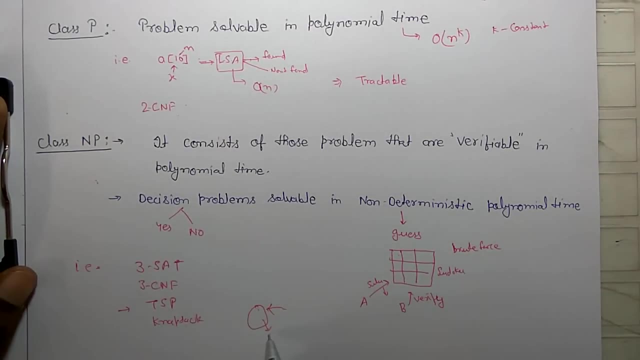 There was a bag And in that you have to collect Maximum price, Or whose weight is more, Or the value is more, That you have to collect W1, W2, W3. There are many weights In which you have to collect. 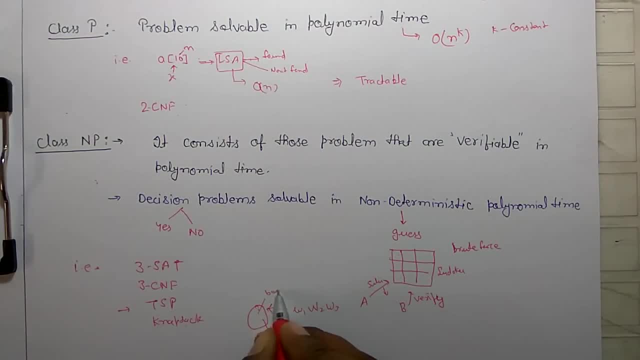 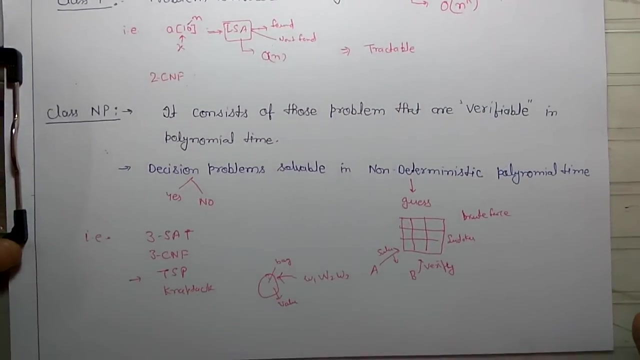 Maximum price value In this bag. So knapsack problem was In this. you perform through guess. That is also considered as NP class problem. So this is difference between P class and NP class. So there is some another terms: NP complete. 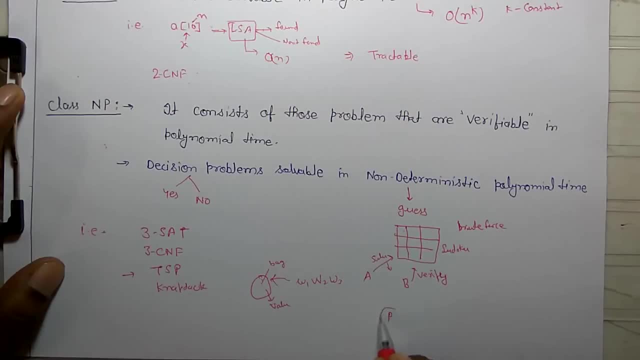 So what is NP complete? This is P class problem And There is NP class problem. There is some NP hard problem And What is its conjunction? NP, complete. So what is NP hard problem? There are some problems Which you can design algorithm. 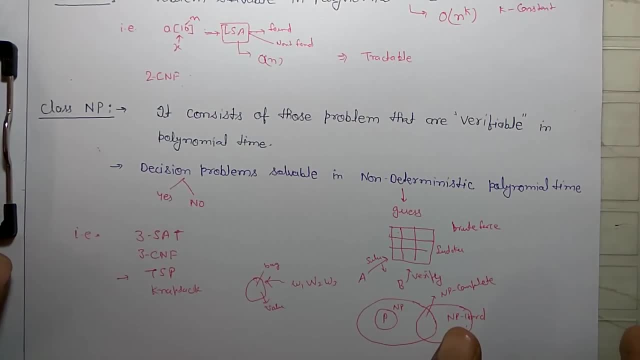 But Maybe it takes too much time And it is not feasible. That is very hard to solve those problems That we consider as NP hard problem. I mean, for example, In case you have Any computer And you have given some instructions in it. 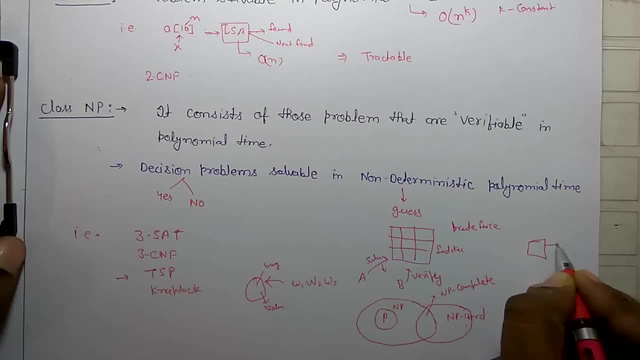 And that computer That Any instructions Execute in 20 milliseconds And, For example, Scheduling problem, You have to do job schedule. So if you have 10-12 jobs, 10 jobs In this computer, You have to schedule.